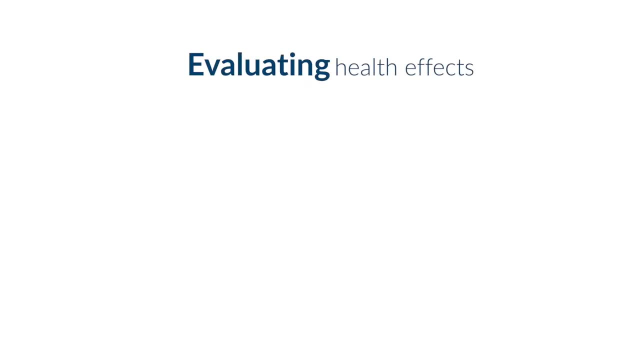 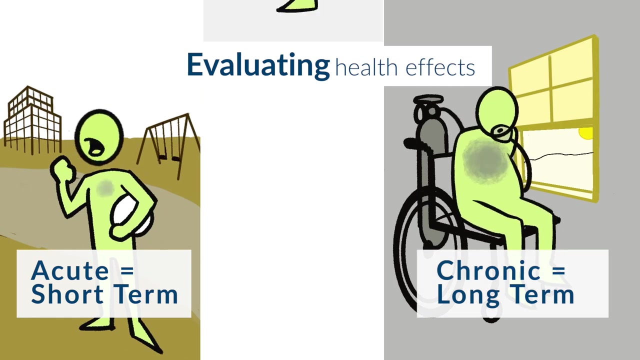 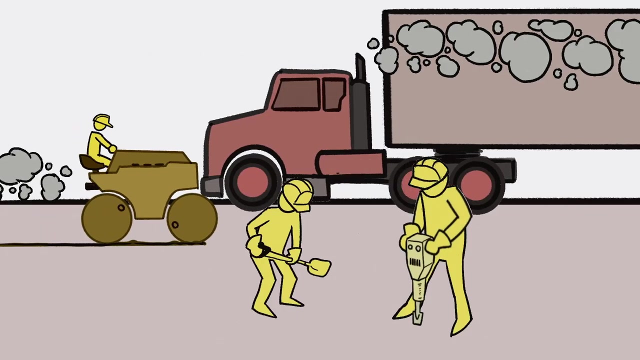 is 72% white. There are two ways health effects are evaluated in terms of how long air pollution exposures last. The first is short-term or acute health effects from immediate exposures. The second are long-term or chronic effects that may last for years. Acute and chronic exposures may occur at the same time. Both types of 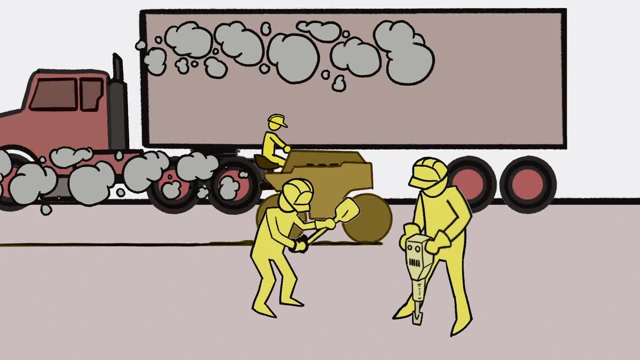 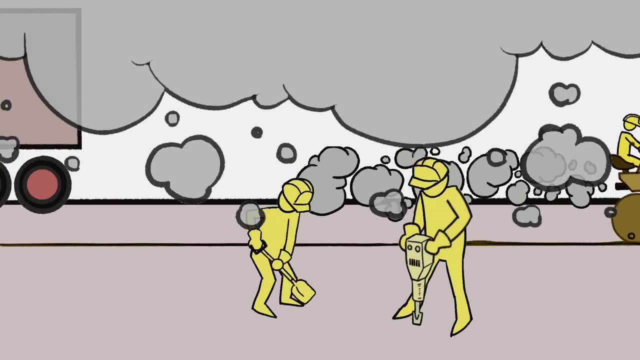 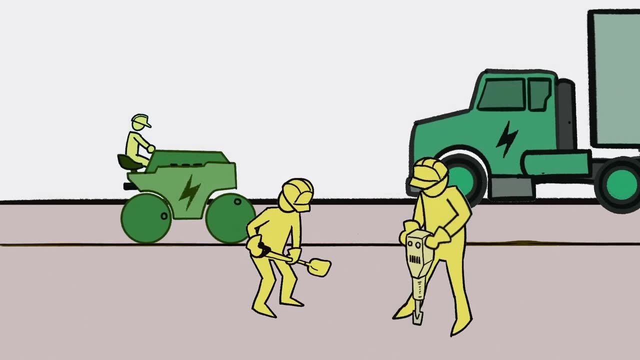 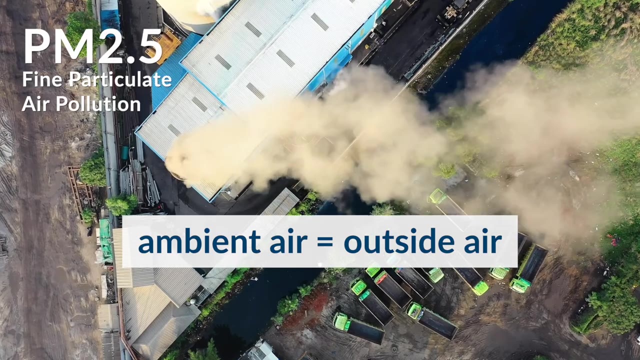 effects may be compounded by working outdoors and living near sources of air pollution such as industrial facilities or roadways. Chronic health effects of air pollution take more time to develop and may not be reversible, whereas acute health effects of air pollution may improve if exposure is reduced. Ambient fine particle air pollution is known as PM2.5. 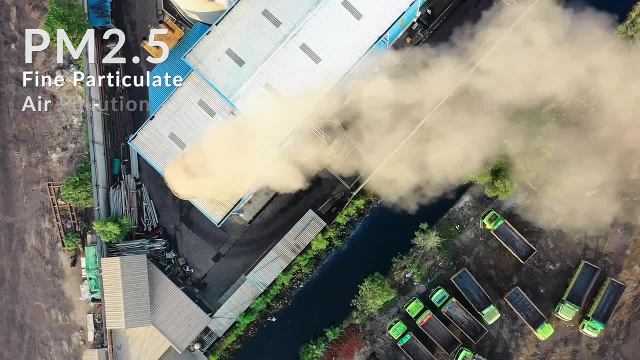 Exposure to PM2.5 is the largest environmental cause of human mortality. The health effects of exposure to potential air pollution may increase if exposure is reduced. The exposure to PM2.5 is the largest environmental cause of human mortality. The health effects of 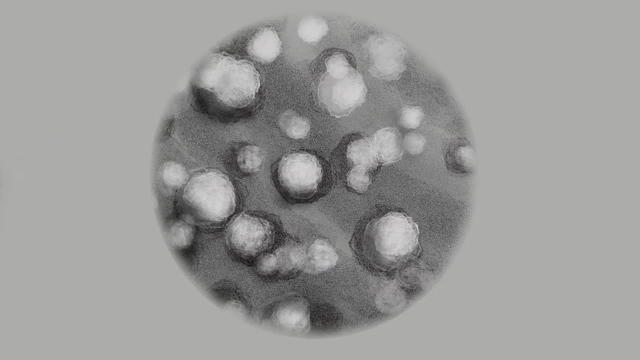 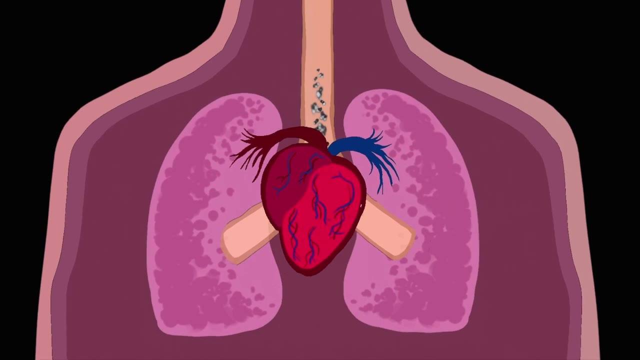 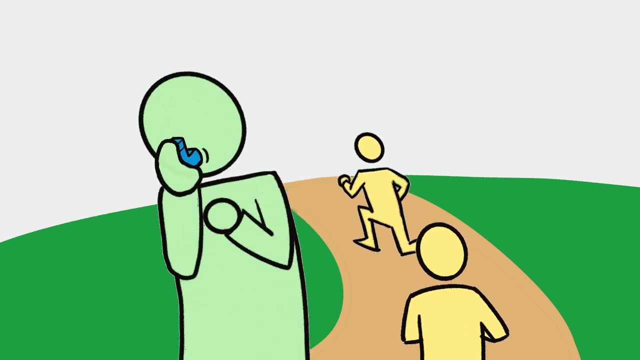 MC2.5 may increase if the physical activity against PM2.5 is reduced. The host었어요 or present daily nature model of impact in PM2.5 into PM2.5 may help raise amone dose per year. Health effects from long-term exposure to particulate matter include increased severity. 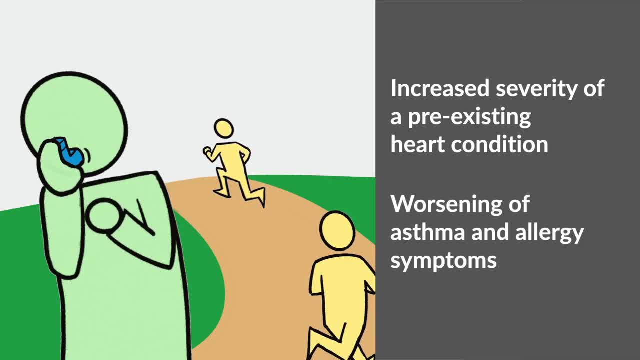 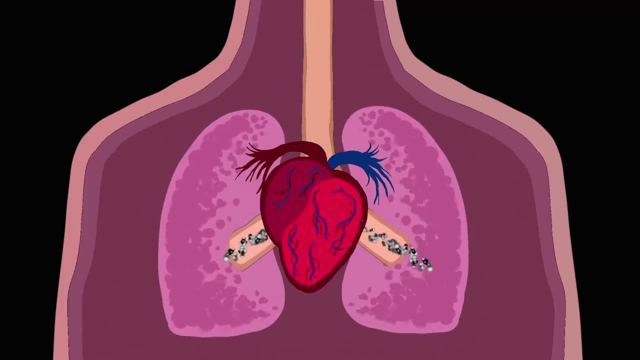 of a preexisting heart condition and worsening of asthma and allergy symptoms. Health effects from long-term exposure to particulate matter include increased severity of a preexisting heart condition and worsening of asthma and allergy symptoms. Health effects include increased risk of heart attack and heart disease. 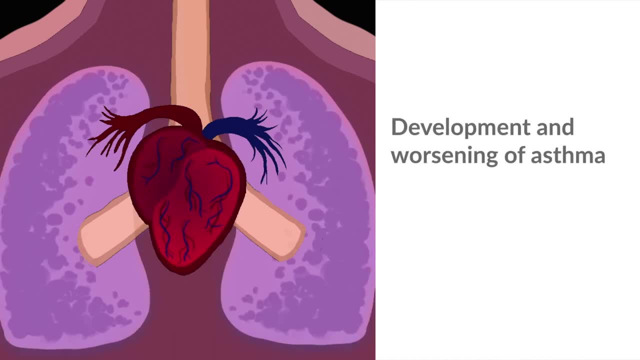 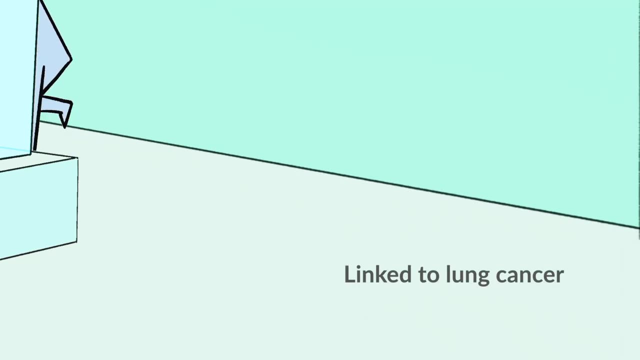 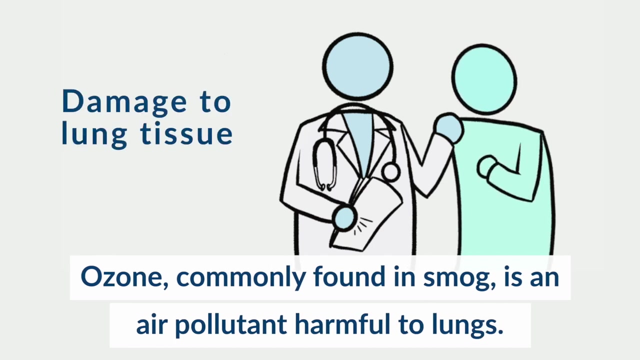 impaired lung function development in children, the development and worsening of asthma and death. Long-term exposure to particulate matter has also been linked to lung cancer, Symptoms of ground-level ozone, including coughing, worsening asthma symptoms and damage to lung tissue. 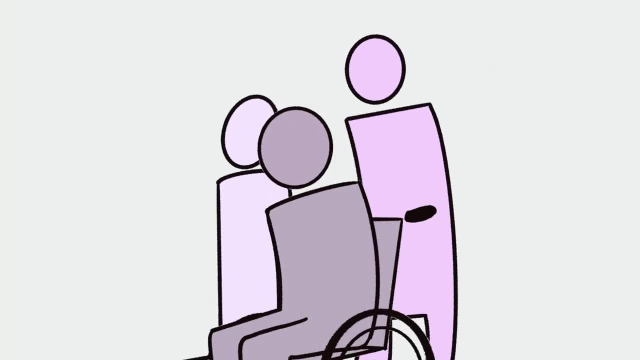 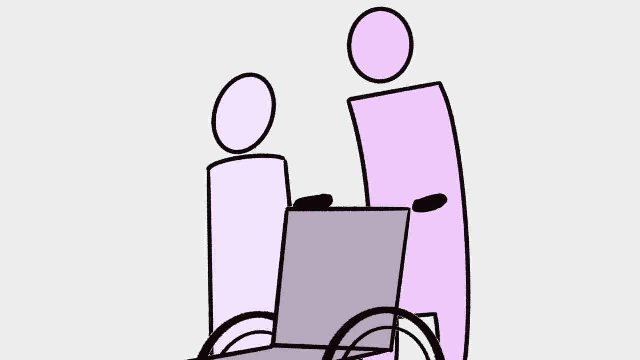 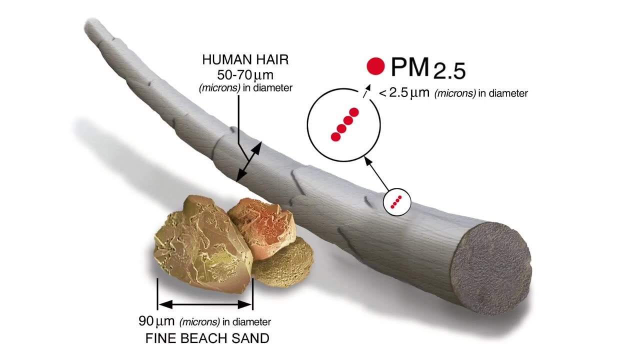 People who have pre-existing respiratory problems may experience increased severity of their symptoms, possibly leading to premature death with repeated long-term exposure. People who exercise or work outside during periods of high ozone are more likely to develop symptoms. PM2.5 and ozone are two of a small number of air pollutants.